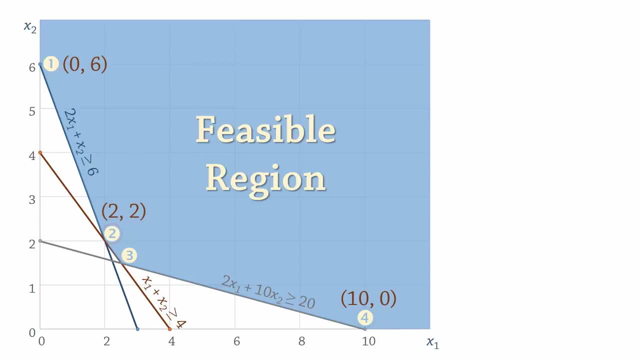 We can also see here that they are 2,, 2 at point 2.. For point 3, we can solve the two lines simultaneously. Multiplying the first equation by 2 and subtracting from the second, we have x2 equals 1.5 and x1 equals 2.5.. Plugging these points into the objective function. 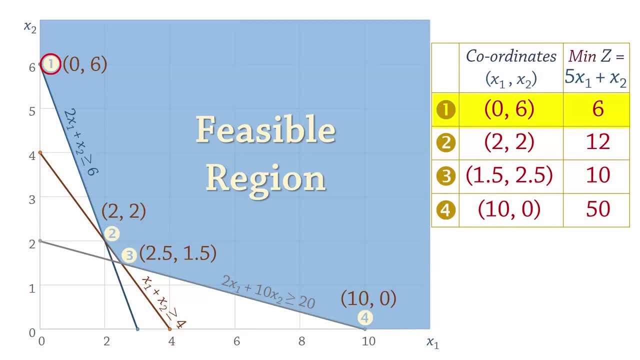 we see that point 1 provides the minimum value of the objective function. So the optimal solution, of course, at point 1, with x1 equals 0 and x2 equals 6.. And the optimal objective function value is 6.. Now for standard form, Since these are all greater than constraints. 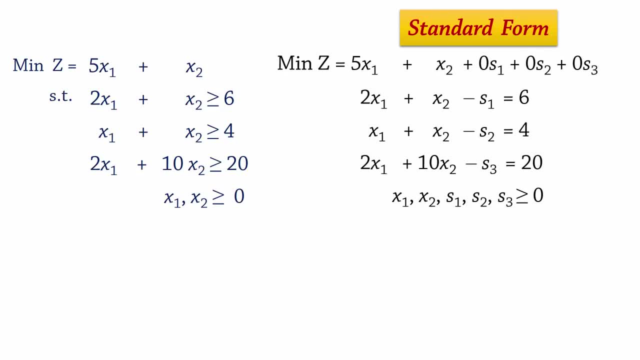 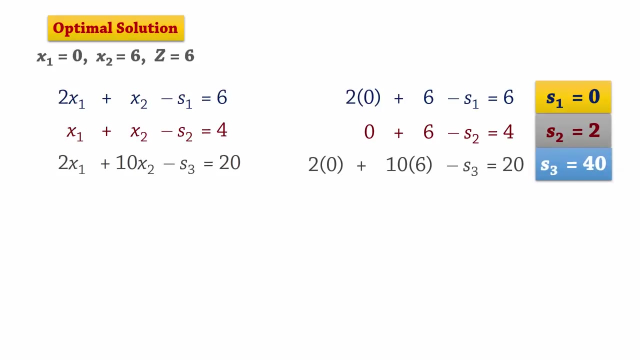 we introduce surplus variables for the three constraints by subtracting s1, s2 and s3 from the left side and changing the inequalities to equalities, Substituting the optimal solution, we have surplus values: s1 equals 0, s2 equals 2 and s3 equals 40.. 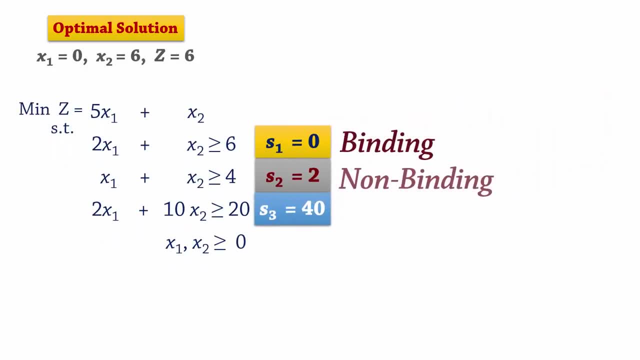 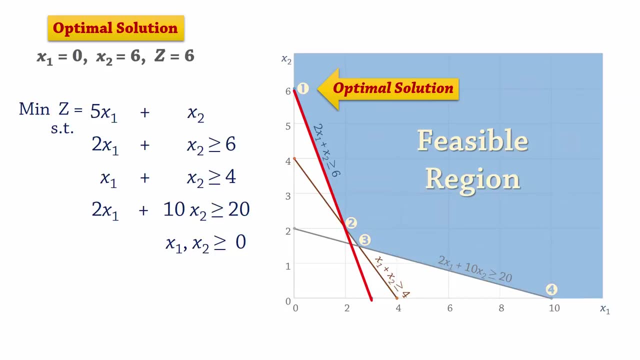 As a result, only constraint 1 is binding because it has a surplus value of 0.. And on the graph we can see that of the three constraints, only constraint 1 touches the optimal solution point. Let's now calculate shadow prices for the constraints. 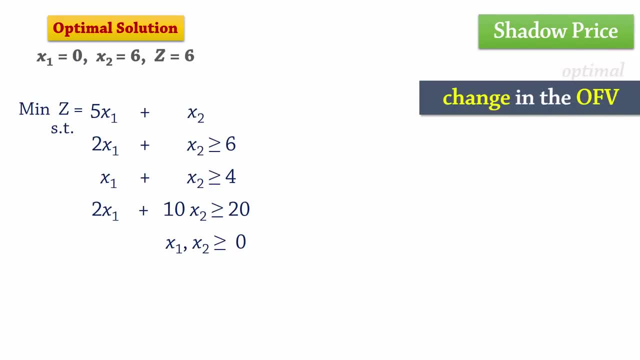 Shadow price here is defined as the amount of change in the optimal objective function value per unit increase in the right hand side of a constraint. So for the first constraint we want to increase the right hand side from 6 to 7 and then determine 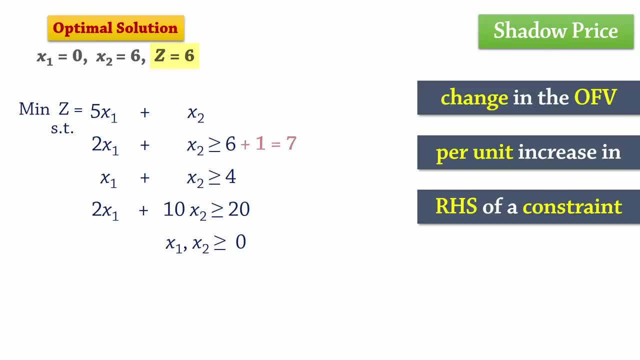 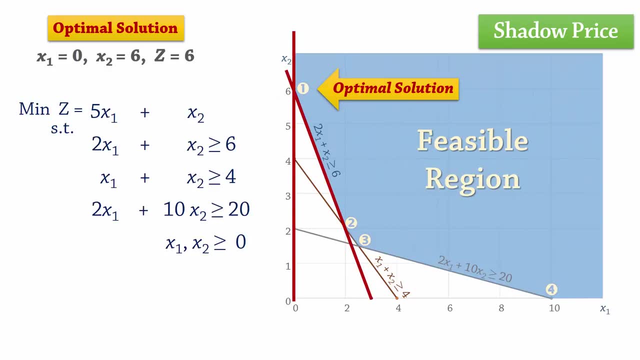 the amount of change in the objective function value As a result. Recall that the optimal solution occurs here, at the intersection of these two lines. So the binding lines are x1 equals 0 and 2x1 plus x2 equals 6.. 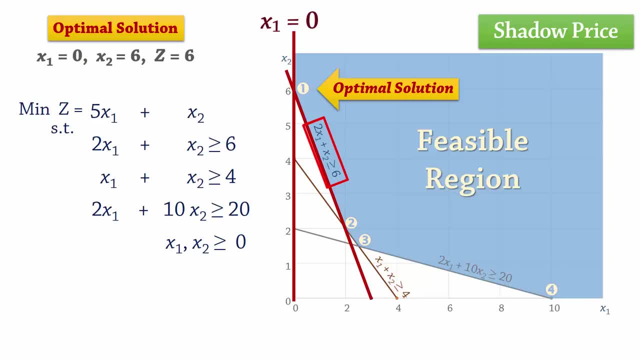 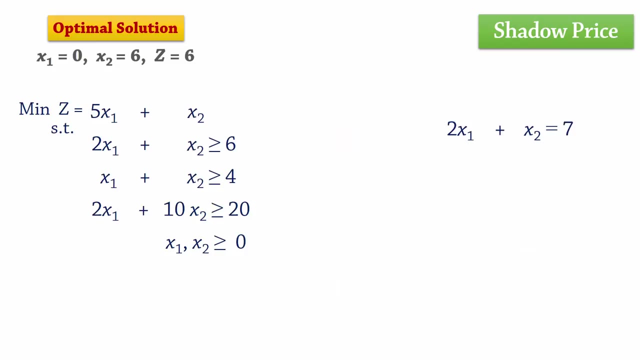 When calculating shadow prices for a constraint, graphically, we increase the right side of the constraint by 1 and solve its equation simultaneously with the equation of a binding constraint. So for constraint 1, we increase its right hand side to 7, and solve it simultaneously with X1 equals 0,. 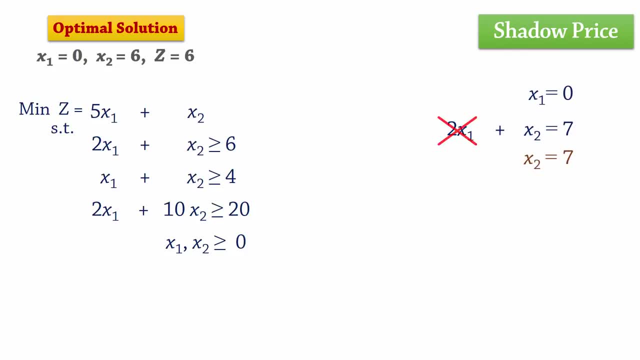 since X1 equals 0, X2 equals 7.. So the objective function value is 7.. We then subtract the old objective function value from the new one to obtain a shadow price of 1.. For constraint 2, a unit increase in the right hand side gives 5,. 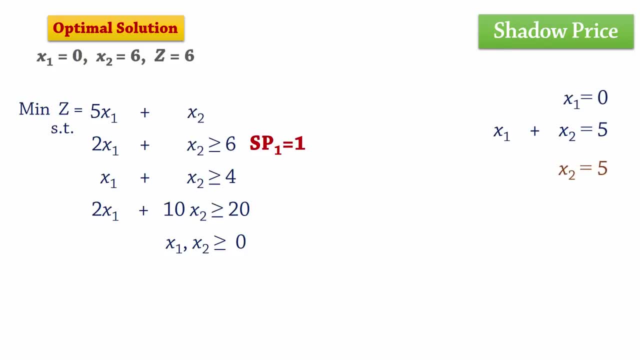 and solving it with X1 equals 0 gives X2 equals 5.. So we have a new objective function value of 5, and the shadow price is 5 minus 6, which gives negative 1.. But wait a minute. We stated a moment ago that the second constraint is not binding. 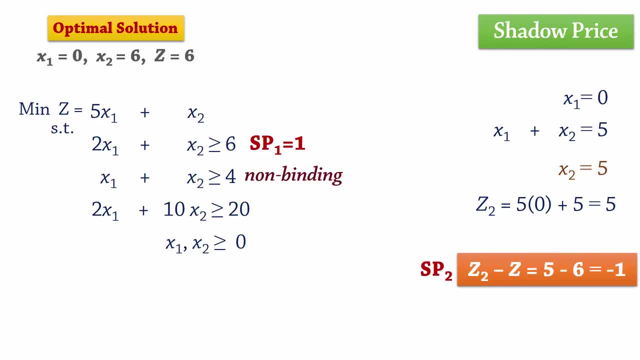 Then by definition it should have a zero shadow price. That is, if a constraint is not binding, it will have a slack or surplus greater than zero and should also have a zero shadow price. So something must be wrong here. The shadow price should be zero. 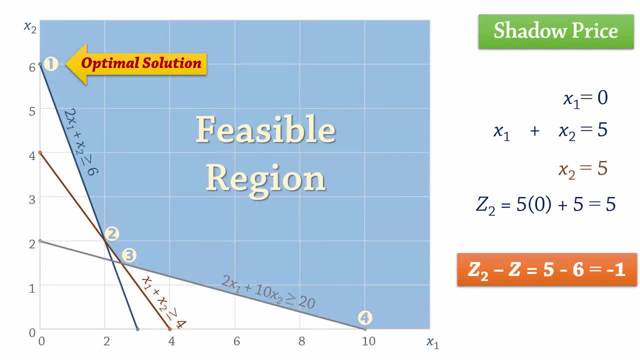 Let's take a look at the graph to see where the problem lies. If we increase the right side of this constraint by 1,, we have this new feasible region. The point 0,5 occurs here, which is outside the feasible region. Therefore it cannot be a new optimal point. In essence, the optimal solution remains here at 0,6.. 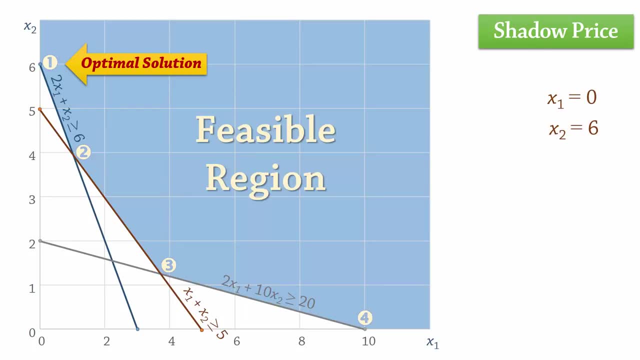 Note that if you have solved it simultaneously with the first constraint here, which is also binding, your solution will be 1,4 here with an objective function value of 9,, which is also not optimal. Therefore, the optimal solution remains at 0,6 and the objective function value has not changed. 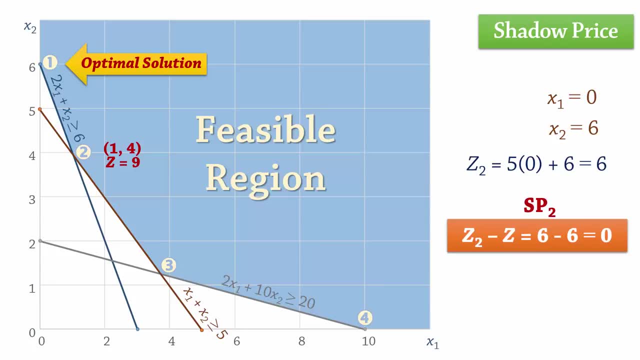 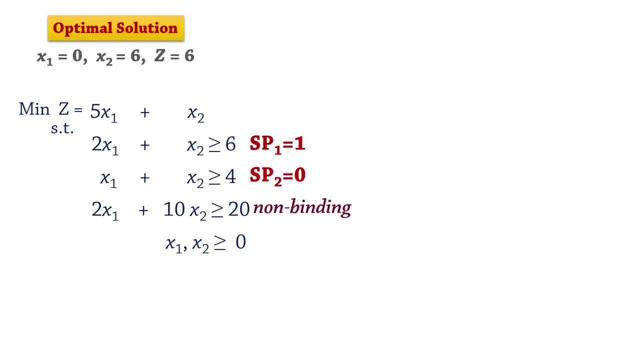 So the shadow price for constraint 2 is still zero. Consequently, we don't need to bother calculating the shadow price for constraint 3.. It is also not a binding constraint, so it will have a shadow price of zero as well. We can see here that constraint 1 is binding. It has a non-zero shadow price and a surplus of zero. 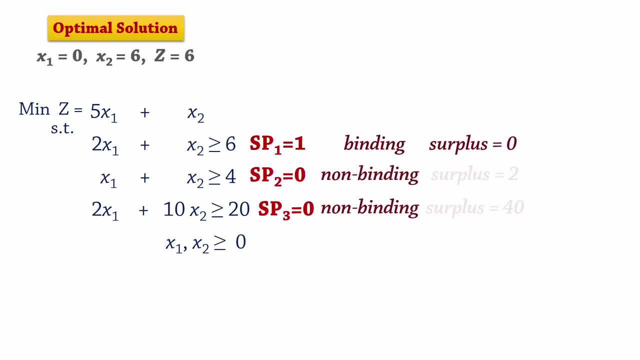 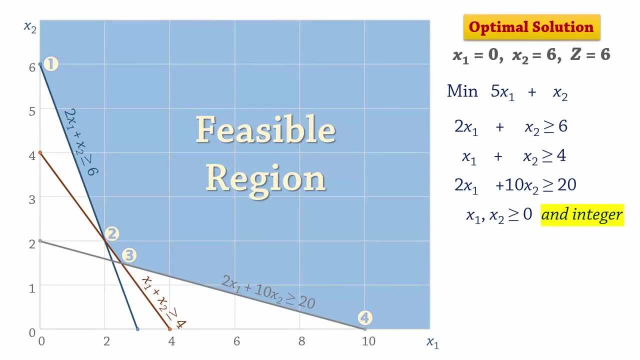 While constraints 2 and 3 are non-binding, with zero shadow prices and non-zero surplus values. Now, if x1 and x2 are required to be integers, then the feasible region is a collection of dots, Since the optimal solution we obtained earlier, which we now call LP relaxation solution. 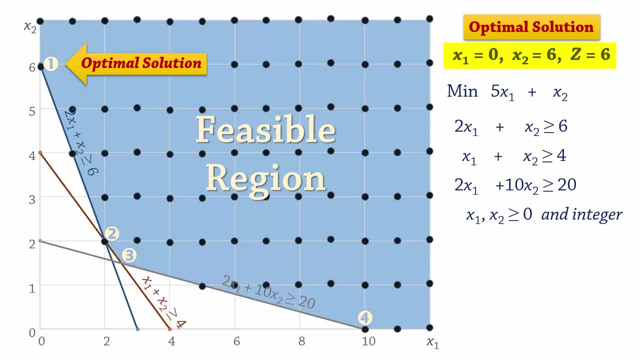 is already integer, then it is also the optimal solution to this integer problem. And that concludes this video. Thanks for watching.